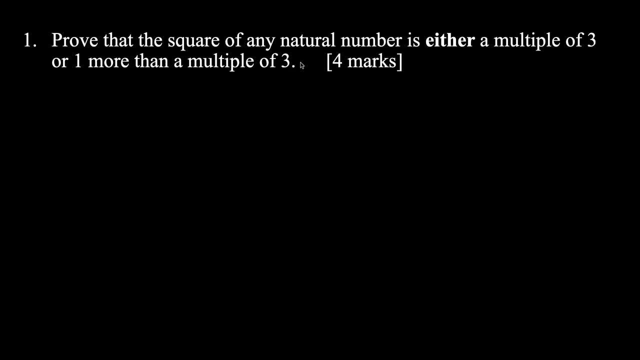 that it's a multiple of three or one more than a multiple of three. we want to represent the natural numbers somehow in terms of multiples of three. So let's firstly look at a list of numbers from one to nine and let's consider how these numbers relate to multiples of three. 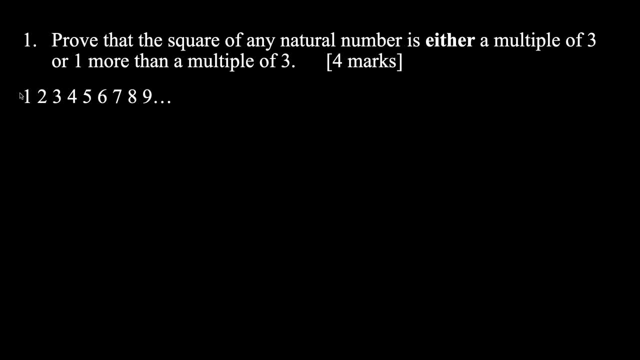 Well, on, we can say, one more than a multiple three. zero is a multiple three. right zero times three is zero. Two is one less than a multiple of three. three is, of course, a multiple of three. four is one more than that. five is one less than a multiple of three. six, two times three. seven is one more than that. 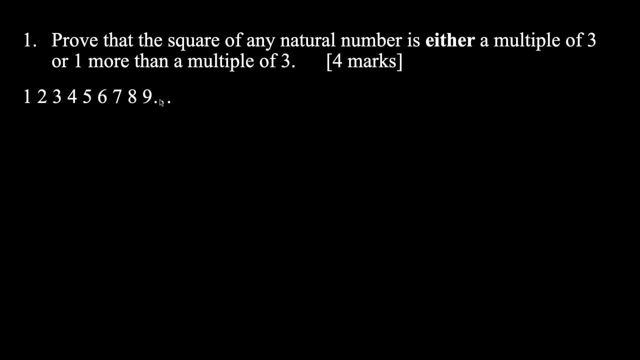 eight is one less than a multiple of three, and then we're again back to three times three. so what am i getting at here? well, we can represent any natural number as either a multiple of three, one more than a multiple of three or one less than a multiple of three. so that's the key observation. 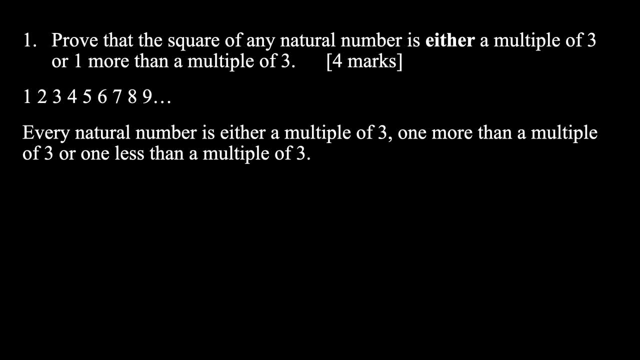 you need to make here in order to answer this question. it is difficult coming up with these observations, but the the clue is usually in the question. if they're talking about things like natural numbers to do with three, think about how you can represent numbers, the natural numbers, in. 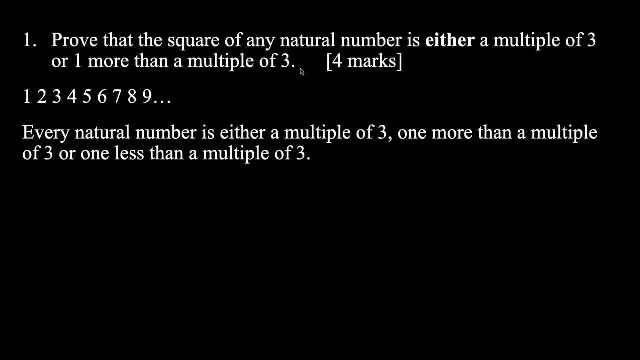 terms of, in this case, multiples of three or whatever number they're talking about in the question. once we have this observation, it should be fairly straightforward from here so we can say that we can represent all natural numbers as either 3k, so that's a multiple of three, 3k plus one. 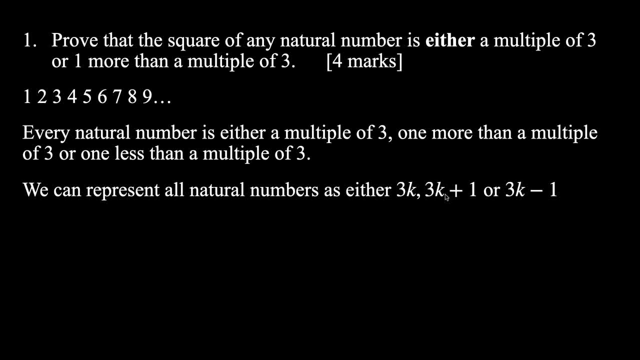 or 3k, take one. these are the algebraic expressions representing this observation we've made. okay, let's consider, firstly, the cases where we have either a number greater than a multiple of three or less than a multiple of three, and we can do those in one go, so we can write. 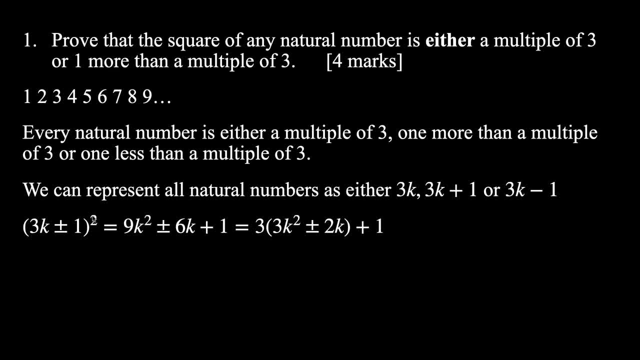 3k, plus or minus one squared, and we'll see what we get. so, expanding these brackets out, this would be 9k squared, plus or minus 6k, depending on which sign you use, and then plus one. it's always going to be a plus one. whether we have plus or minus in there, it's always going to be a plus one. on the 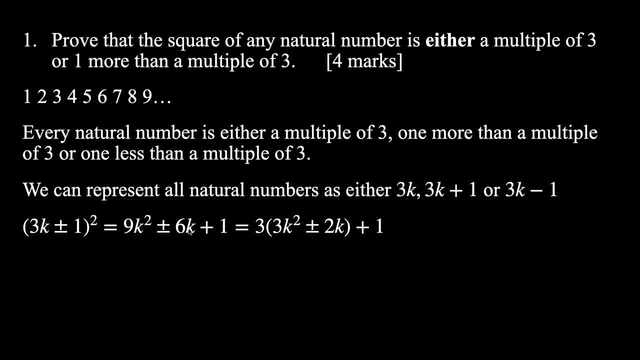 end, and then this 9k squared plus or minus 6k. we can factorize the three out of that and we get three multiplied by 3k squared plus or minus 2k plus one. this expression represents a multiple of three plus one, so this is always one more than a multiple of three, that's. 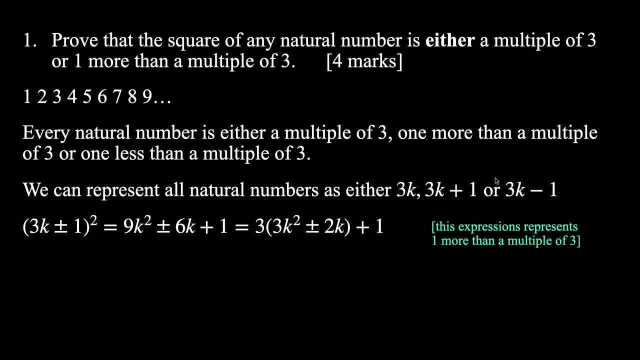 what that expression represents. okay, so that's the case where we've got a natural number and it's either one more or one less than a multiple of three. what if we have a multiple of three and we square that? well, that's pretty straightforward, right? so we'd have 3k squared, that's 9k squared. 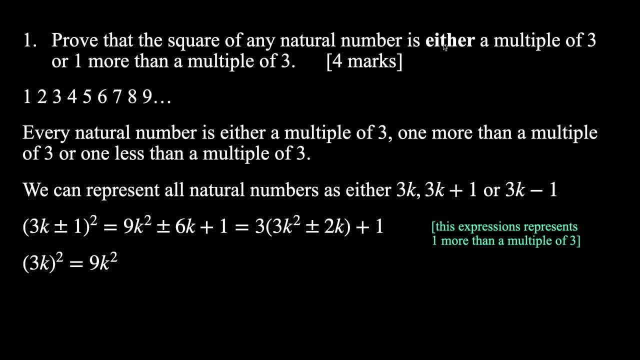 that's clearly a multiple of three. go back to the question. we need to show it's either a multiple of three or minus 6.. of three or one more than that, and we've done that, with that working out there. so we can finish our proof by saying: therefore, the square of any natural number is either a multiple of three or 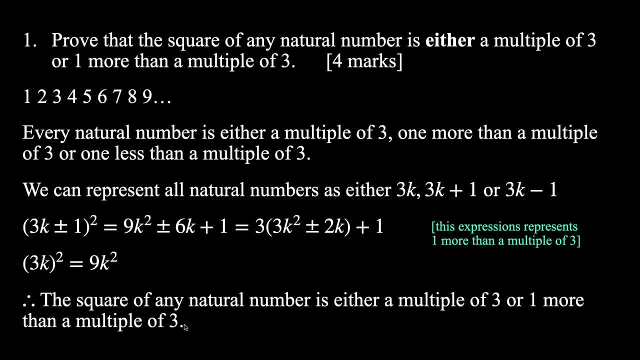 one more than a multiple of three. so there you go. that's about all the working out you needed for that question. i don't want to make it seem like this is obvious. making these types of observations is not easy, but it does come with practice once you've done a number of these algebraic proof. 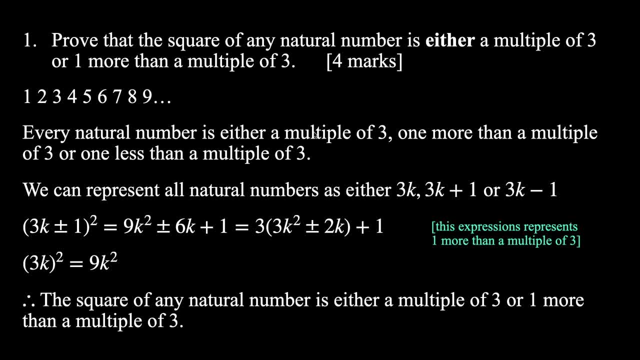 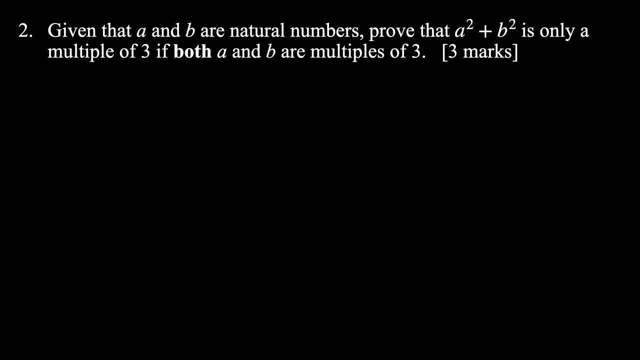 questions you do sort of see like how to begin them and the types of methods you need to use. so i would say with practice this does get easier. question two now that first question was an actual exam question, not written by me. these next two questions i made up so they might not be quite. 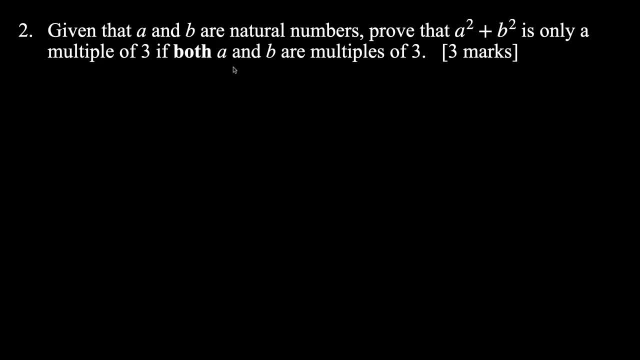 as good as the first one, but i hope they're still useful. so this question says: given that a and b are natural numbers, prove that a squared plus b squared is only a multiple of three if both a and b are multiple of three. think about what we just proved. we proved that the square of any natural number is: 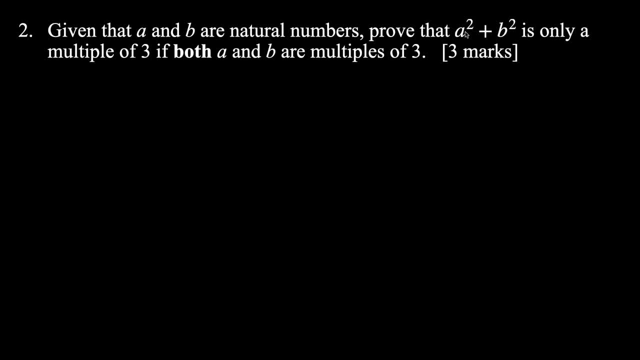 either a multiple of three or one more than that. so what are our options here for a squared plus b squared? well, a squared could either be a multiple of three or one more than that, and the same with b squared. so let's firstly consider the case where they're both not multiples of three. so 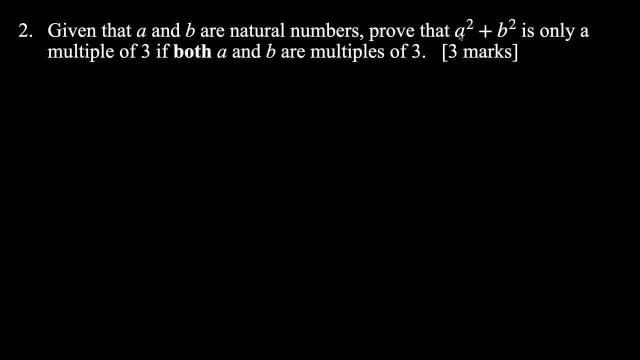 they could be both one more than or one less than a multiple of three. so let's consider that case. we had, for example, three p plus or minus one, and then three q plus or minus one. we square those now they're both going to be, as we just proved, one more than a multiple of three. so what? 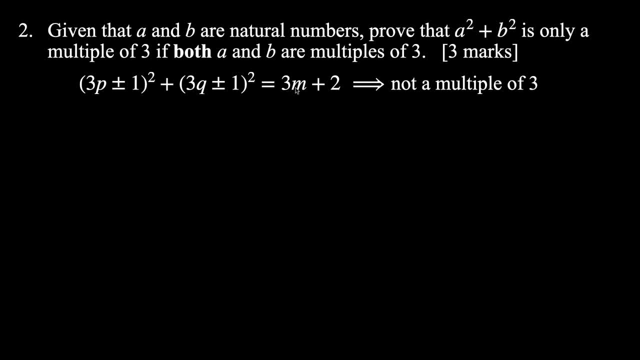 would the result be then? we'd have a multiple of three, which i've said is 3m. you can use any letters here. by the way, it doesn't really matter what letters you use. that's just saying this number will be a multiple of three, but we'd have plus two on the end, right, so we'd have a multiple of three. 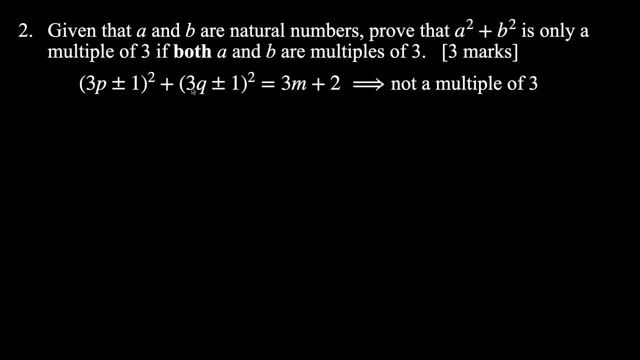 right, because both of these are one more than a multiple of three. we need to add those two ones together and we get plus two, in other words a remainder of two, and this is clearly not a multiple of three. what are our other options? well, we could have a being one more or one less than a multiple. 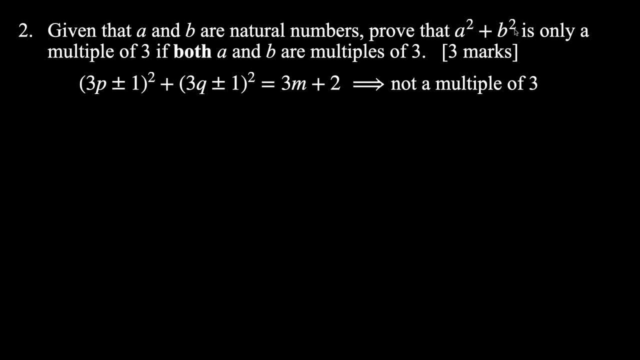 of three and then maybe b is a multiple of three. so let's consider that option. so a we could represent as three, p plus or minus one squared, and then b is a multiple of three. so that's three q squared, but here a squared is going to be a multiple of three plus one. okay, so when we add: 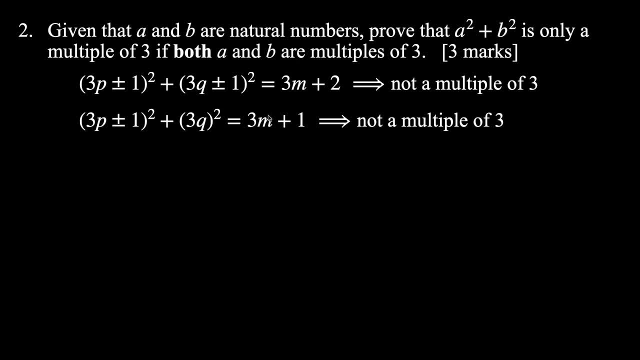 these together, we're going to get a multiple of three, but we're always going to have a remainder of one, which i've represented as 3m plus one. so because we have that remainder of one on the end, it's never going to be a multiple of three. okay, now the only other option that we haven't. 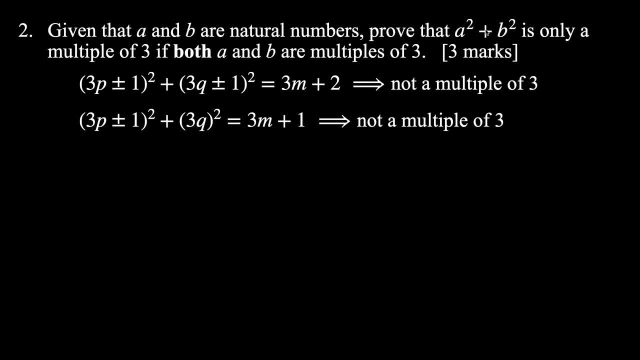 considered yet is if a and b are both multiples of three, and if we add two multiples of three, clearly the result is going to be a multiple of three, and in fact that's what the statement says, right? so this is enough to say that, therefore, a squared. 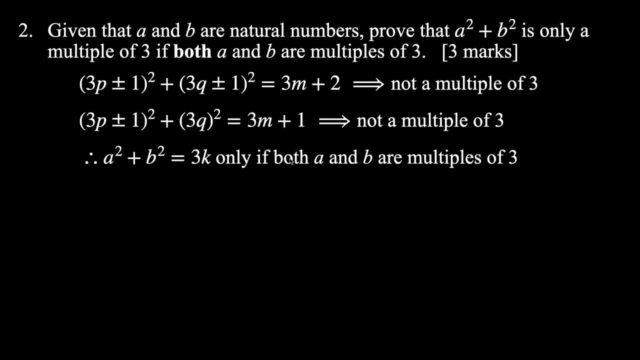 plus b squared equals a multiple of three only if both a and b are multiples of three. okay, so that's how you could answer that type of question. the last question was an always, sometimes never proof. so this question says: richard states that a squared plus b squared is only 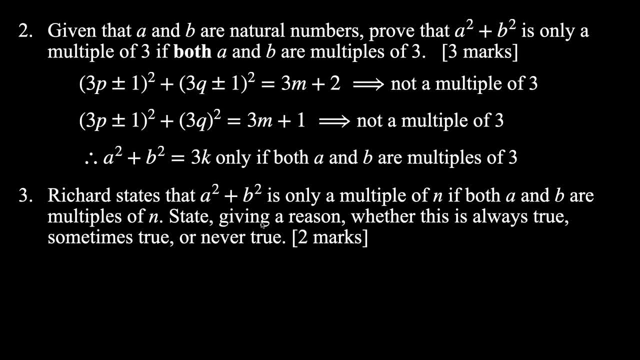 a multiple of n. if both a and b are multiples of n, state giving reason whether this is always true, sometimes true or never true. i put two marks here because there's a bit of interpretation that you need to do in the question, but once you've interpreted the question correctly, i 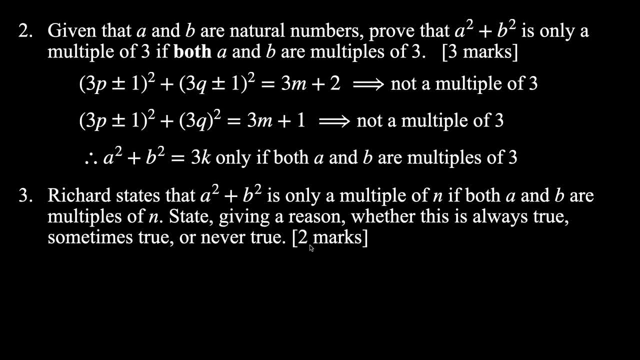 don't think it's really too challenging. so what we want to do here is to use a counter example. so can you think of two numbers, if you square them and add them, that the result is not a multiple of the numbers you used? so let's pick, you know, the first two numbers, the first two counting. 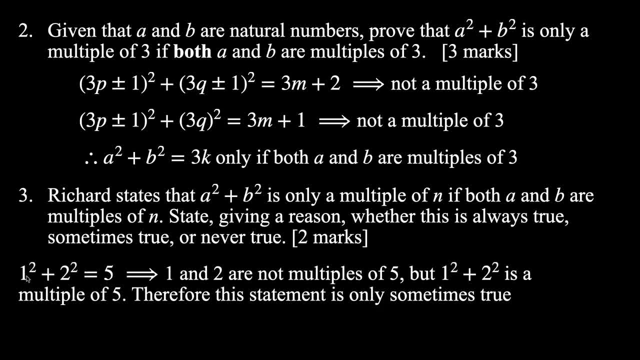 numbers one and two. so one squared plus two squared is five. one and two are not multiples of five, but one squared plus two squared is a multiple of five. so let's read this statement again. richard states that a squared plus b squared is only a multiple of n if both a and b are multiples of n. 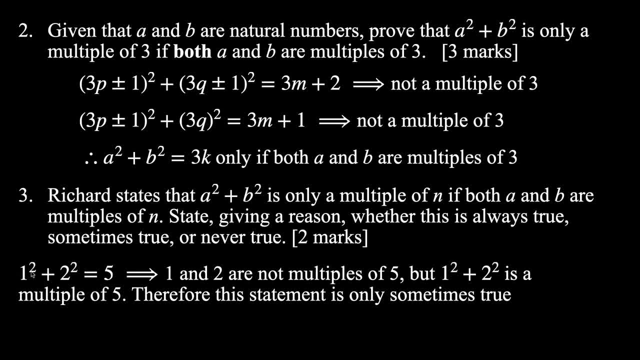 so what if we said n was five? well, one squared plus two squared is five, but a and b, in this case one and two, are not multiples of five. so clearly, for this example, this statement is not true. okay, so this therefore: this statement is only sometimes true, for example, if n is five. it's not true, but it is. 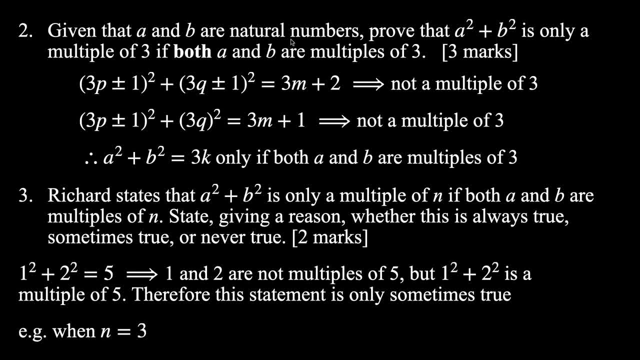 true if n is three, as we have shown in question two. so for that question you just needed to give a counter example. there are many other examples you could give. for example, if you did three squared plus two squared, what would that be? that would be nine plus four, that's thirteen. nine and four are not multiples. 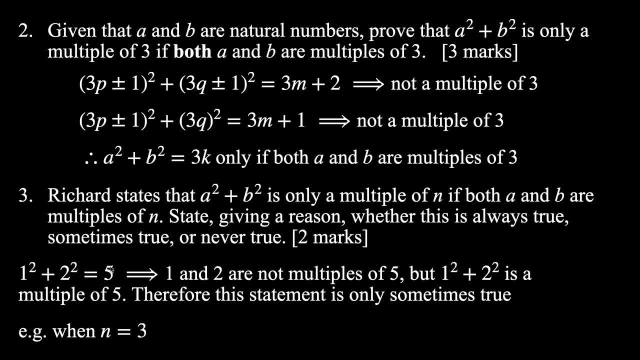 of thirteen, but you get a result which is a multiple of thirteen. so that's another counter example. so often it's really useful, when you get these always, sometimes never- questions, to use counter examples to prove that they're not always true. okay, there is some algebraic proof questions. i hope you found that useful. see you in the next one. bye for now, you.